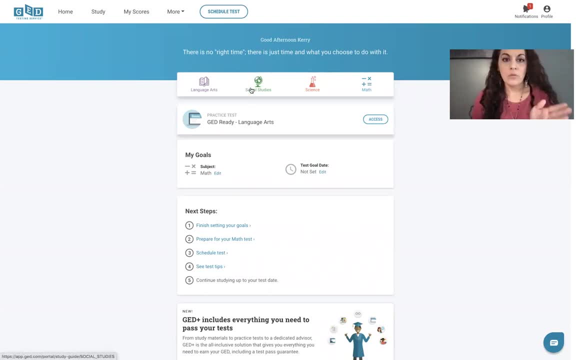 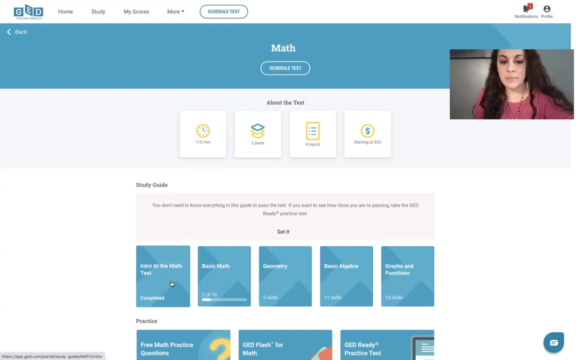 If you click on the subject I'm going to go with math. So if you clicked on that subject here in the top, it gives you some practice questions to kind of go through. But when I was teaching GED or adult education classes, a lot of people wondered: why are these answers already selected? 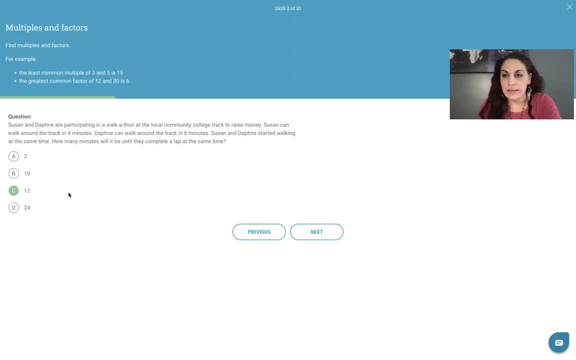 So whenever you click on it, the answers are already selected And it's because this is showing you or explaining, Explaining the skills that are going to be on the math test, the things that you should be studying or be comfortable with to be able to pass that math test with a passing score which is 145 or higher. 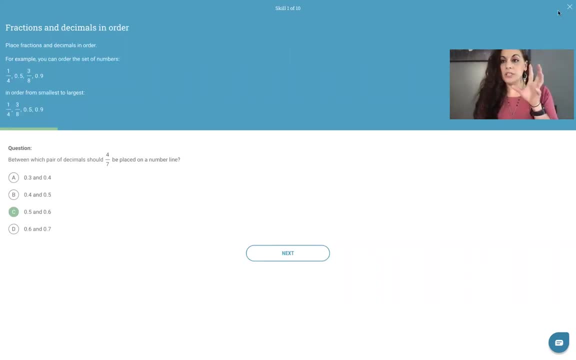 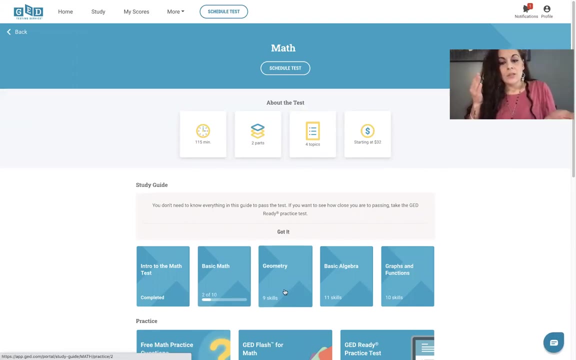 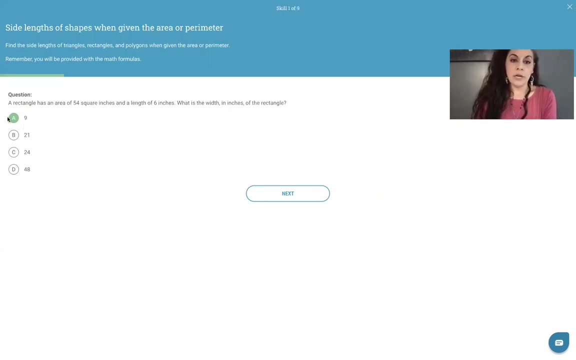 Clicking on it there's different kinds of questions, So it breaks it down by skill in the beginning, but the answers are already listed on there So We can use them. but I want to try to make that. I want to try to make them more beneficial. That's my goal. So, clicking through these, you will see that there's many different things, But once you click on it and if you were to create an account, the answer will already be selected. 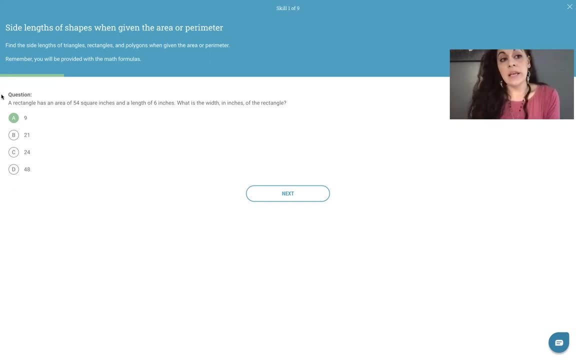 The biggest thing that you can get out of this is reading this top part here. A lot of people miss that. I missed it even as an instructor for a long time And then working the problems backwards. So you know that this is the correct answer. but if you figure out how- 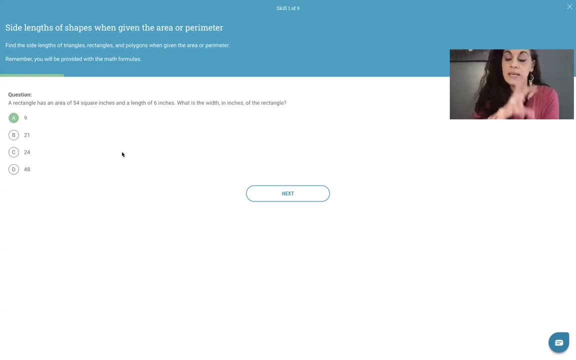 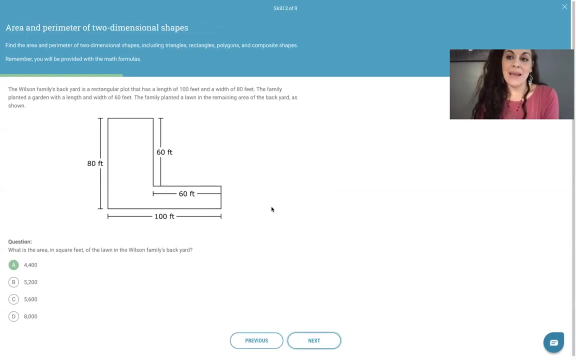 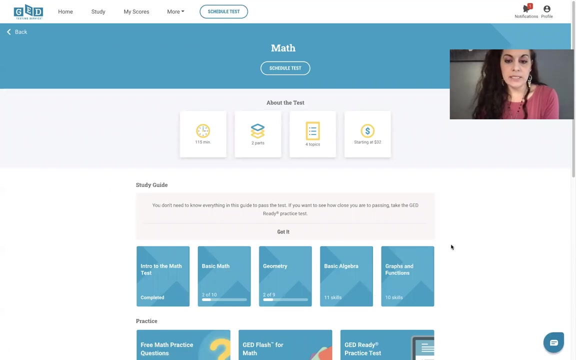 They're using or what they're using to get to that answer. then you can understand the process. A lot of these questions are very simple. For the math test it is more. So it's 55% algebra in the test, So it breaks it down. 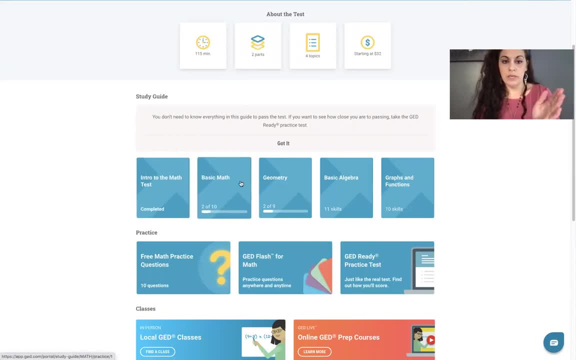 I mean in each category: basic math, geometry, basic algebra, basic algebra. So it's 55% algebra, but it's 7th, 8th, 9th grade algebra. It's the beginning, rules, order of operation and then it has slope. But most people freak out because they say that I never took algebra. 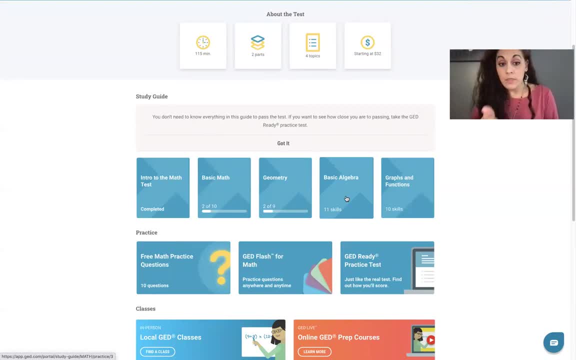 Well, if you're in this class or you're on this website, no, you probably didn't, because you're working toward gaining or growing what you missed out on So studying. Yes, it's algebra, but it's not as bad as what it seems. 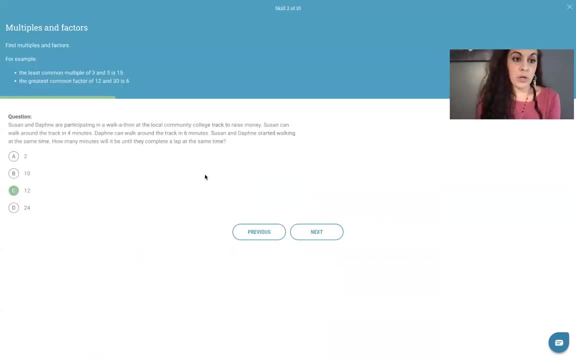 I just want to, on this video, explain one question, just to get it started again, get it posted. I want to find somebody, even if it's one person that this is helping. I spend a lot of time on my own doing whatever I want, but I want to help other people. 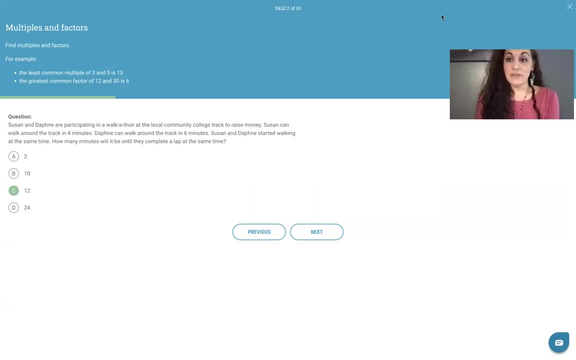 And I enjoy math. So if I can find a way to help people doing something that I enjoy, then I'm winning. right, I am going to, I am on Zoom, I'm recording it, So then I'm going to post that if anybody's curious. 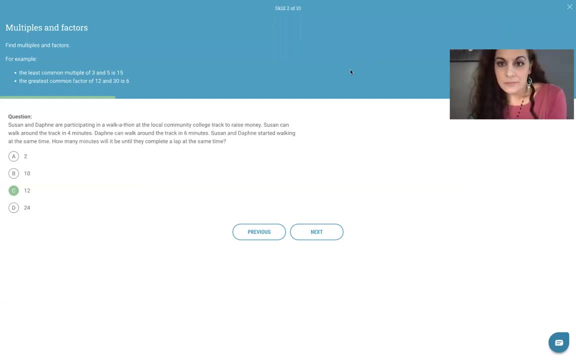 Yes, All right, I'm going to use a marker on the white part here too. So I'm going to use a marker on the white part here too. So I'm going to use a marker on the white part here too For this question. 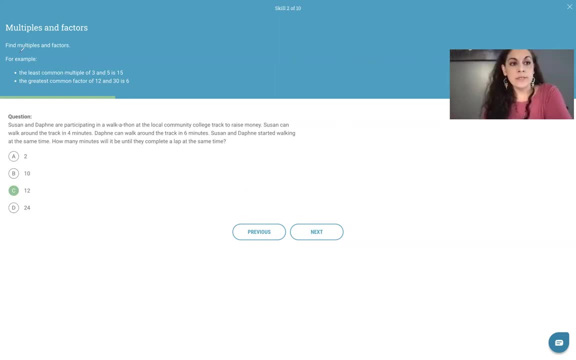 This question. it gives you the scale at the top, multiples and factors. It says find multiples and factors, for example, the least common multiple and the blue didn't work too well on the blue. The least common multiple of three and five is 15, so least common multiple is a strategy that you need to be comfortable with on the test. 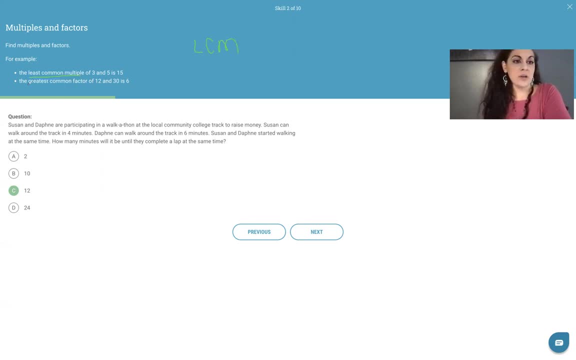 And greatest common factor is also a strategy that you need to be comfortable with on the test. So in this example up here, yes, it gives it, but most of you might not understand where those numbers are coming from or you really have to process it. So it's important to study with other resources as well. So the least common multiple of three and five is 15.. Multiple is when that number is being multiplied up, when it is going higher and higher. So of three and five, least is the smallest. common is the thing that they have the same, So the smallest number that is common for them. 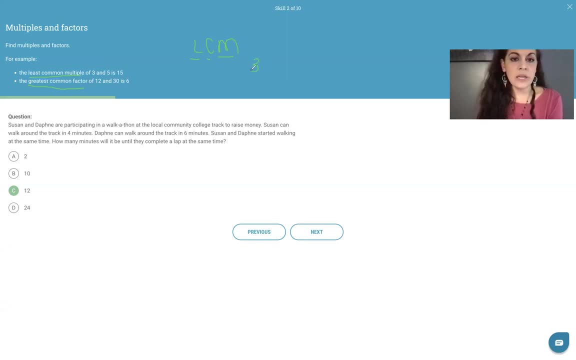 as a multiple. So what I'm going to do is list three and five. This is for the example. not even on that question yet, but then I'll show you what least common multiple is. It says the least common multiple of three and five is 15.. Well, multiples of three. 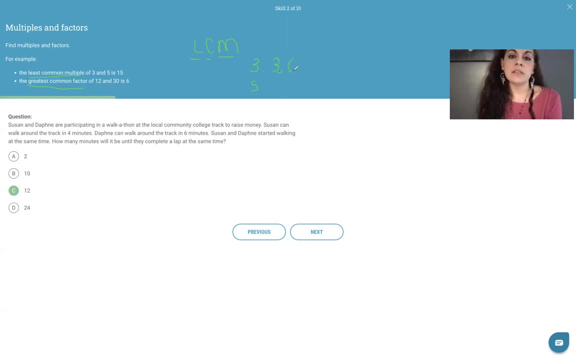 three times one is three. three times two is six. three times three is nine. three times four is 12,. three times five is 15.. I'm just going to list a few of both, Okay, Because we're looking for the least common multiple of three and five. 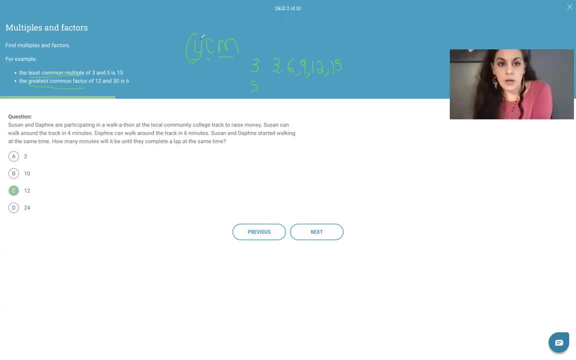 least not just just a common multiple, because it there will be more other multiples, like 30 is a common multiple, but it's not the least common multiple. um here: 5, 10, 15, 15 is the number that is listed first. for both of them that matches 15 is the least common multiple. that's what they're. 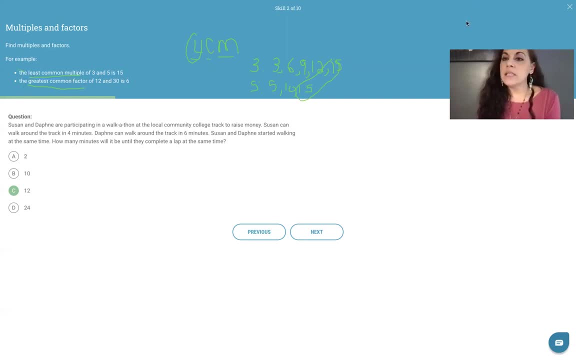 talking about here. and then greatest common factor: um, the greatest common factor of 12 and 30 is 6. notice that that 6 is smaller than those numbers. that word factor is breaking down digits. so we are taking 12 and 30 and listing how. what numbers do i multiply together to get that number 1 times 12? 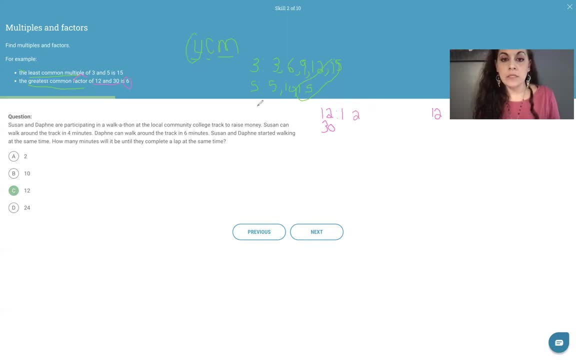 0, 2 times and this is for g, greatest common factor, greatest not least. the other one was least, this one is the greatest. so 2 times 6 and 3 times 4. that's all of the ways that you can get 12, okay, and then 30, 1 times 30. i always go 1 in that number when it's factors. when you're breaking that. 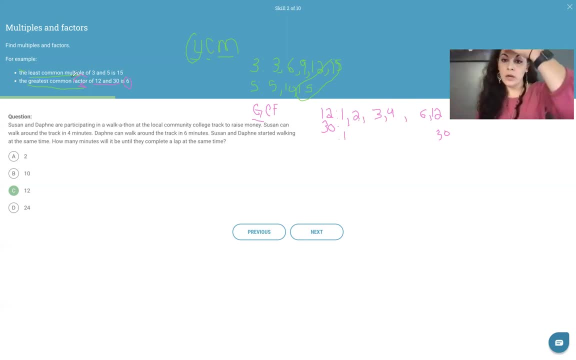 number down. if it's a multivariate, it's a full number. it's a full number. if it's a multiple multiple, then you're multiplying it. You're bringing that number up. So 31 times, 32 times 15.. I'm going to run out of space. 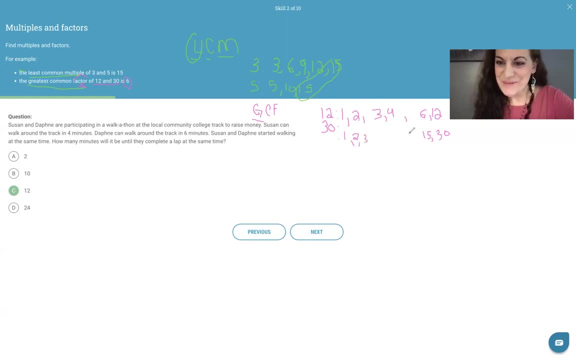 Three times 10.. I wanted to work faster. Does four go into 30?? No, And then five times six. Um, see that one, two, three and six are all common, but we want the greatest six. That is extremely important. Now I'm going to read the actual question and then: 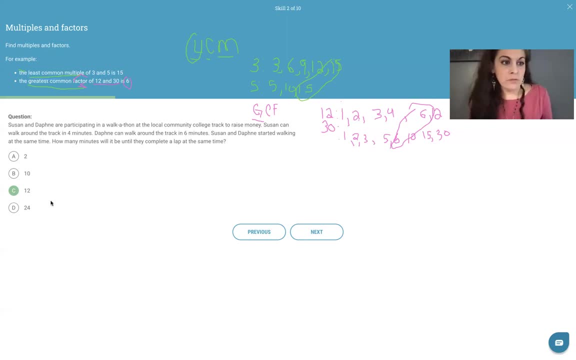 show you how did they get 12?, Because these answers are already answered for you if you're using this to practice. Um, I don't know where that came from. Hi, It's a bunny rabbit for Easter. Susan and Daphne are participating in a walkathon. 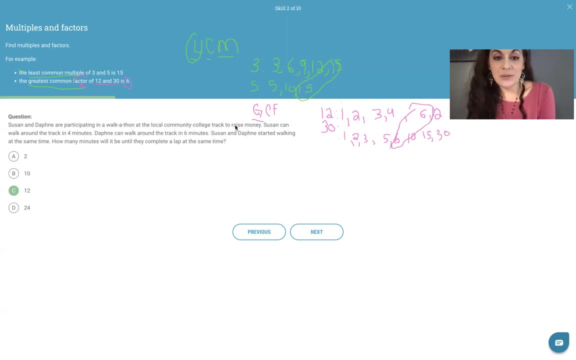 at a local community college track to raise money. Susan can walk around the track in four minutes. Daphne can walk around the track in six minutes. Susan and Daphne started walking at the same time. How many minutes will it be until they complete a lap at the same time? 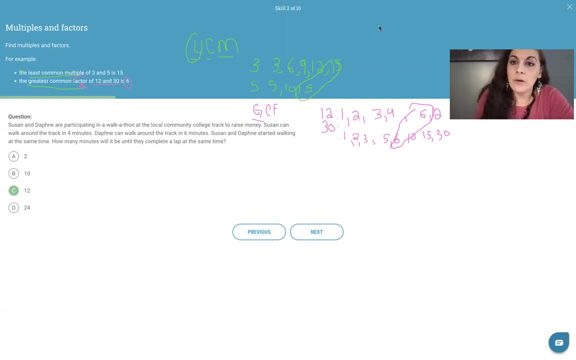 And it is very important when you're doing math, because there's a lot of words. It's like whoa, I thought I was doing math And I only see two numbers in there, or yeah, I see a four and a six. Okay, So remember that on this math test. it is a mathematical reasoning And that is actually. 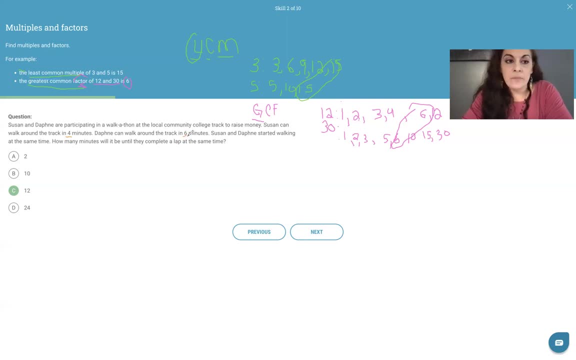 what it says is a math right, Mathematical reasoning exam. You have to take real world situations and be able to reason that reason through them, to come To a conclusion based on using strategies that we learned um, throughout, throughout, education. So, Susan and Daphne, they're running around a track and they don't run at the same pace. 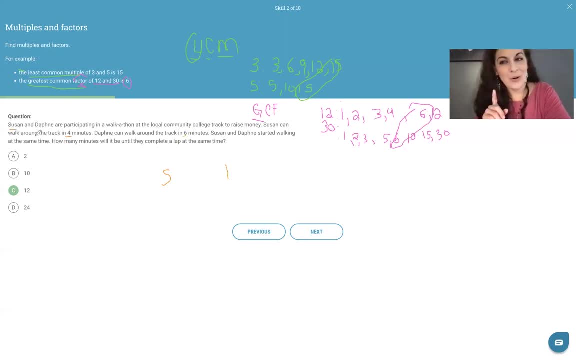 Susan. it says Susan can walk, walk, walk around the track in four minutes. So here we got Susan and we have Daphne, So she can walk around the track in four minutes and Daphne can walk around the track in four minutes. 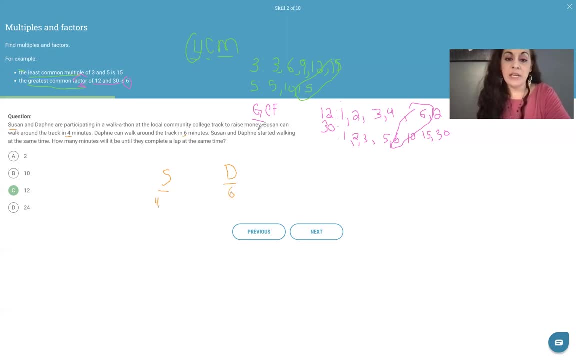 Susan and Daphne started walking at the same time, So they started at zero, zero, um, or at the time clock being zero, zero. How many minutes will it be until if? if she's finishing in four minutes and she's finishing in six minutes, Susan is finishing faster, She's finishing more, She'll. 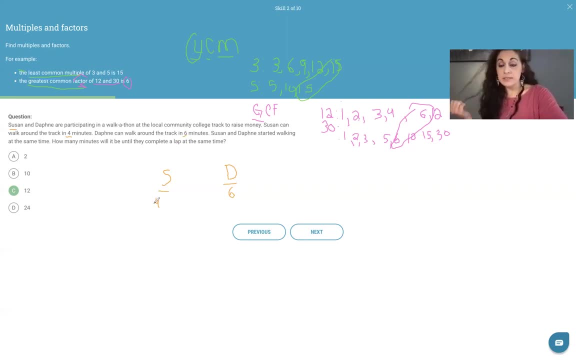 finish more laps. If I can finish a lap in four minutes and she finishes in six minutes, then Susan is two minutes faster than her. So there are several ways that you can process through this question And really you don't have to do all of this. It is important that you're comfortable. 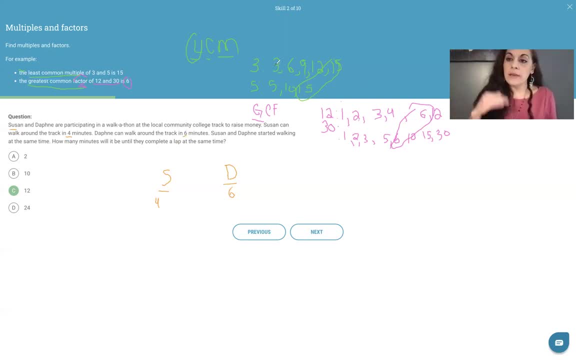 with numbers, or at least adding, to be able to find the next multiple of a number. Um, there's only like five questions on the math test that you will not have a calculator, and you probably won't have a calculator for this one. All I'm going to do is list multiples of four for Susan. So on the first, 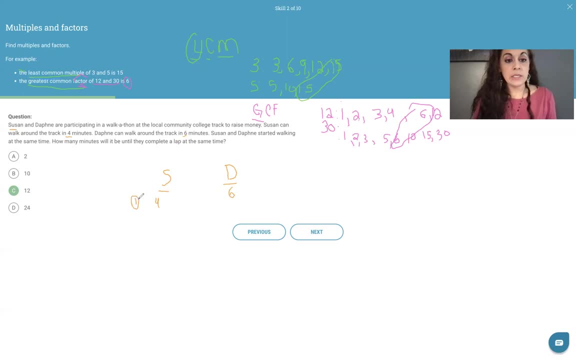 on the first lap, it took our four minutes. On the second lap it's going to take, it would have been eight minutes passed. eight minutes passed during the second lap. On the third lap, it would have been eight, nine, 10,, 11,, 12 minutes: 12 minutes passed. Okay, And notice that this is listing multiples of the 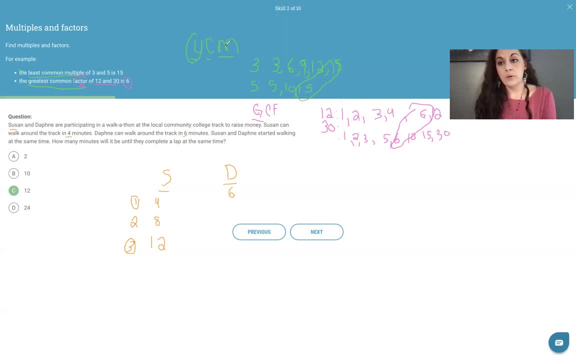 number least common multiple We are finding, we're using that strategy up there- least common multiple To find this. Now I'm going to list multiples of six. The first lap: six minutes. The second lap: 12 minutes. six, 12, six times one is six. Six times two is 12.. Six times three is 18.. Oh, but 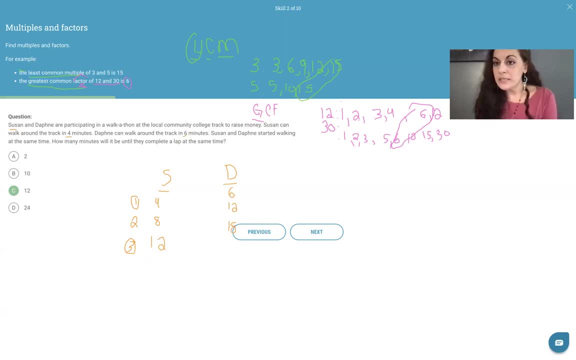 I'm going to stop because I just noticed that I already have a match and I'm looking for the least, the smallest that that is common. So 12 at 12 minutes They would have matched. They would have passed again. So Susan probably would have kept going. 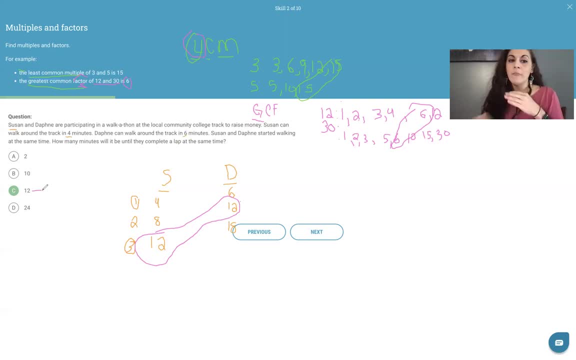 faster, but at 12 minutes they would have passed at the same time, or they they would have completed a lap at the same time. It doesn't say completing the entire race or or walk-a-thon at the same time. That's important. So a lot of us get get caught up in all of these other things because 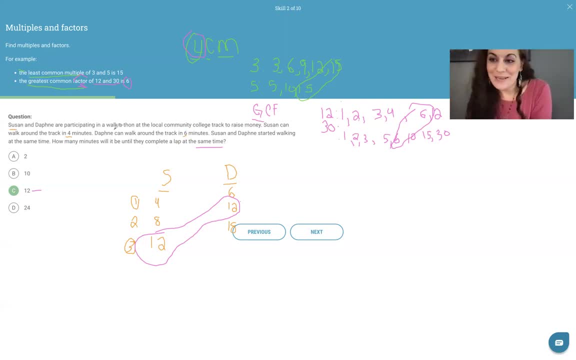 we have ADHD. There's that rabbit again. I'm sorry. Easter, happy Easter. We get caught up in things that we shouldn't be caught up on, We get distracted and you're doing a math test, a math question: focus, just see what is it asking me and then get it right. 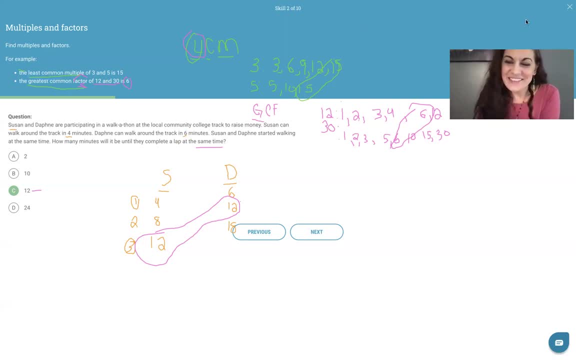 Okay, And that is all I got for this question. So have a nice day. Maybe I'll stop. Okay, Have a nice day.